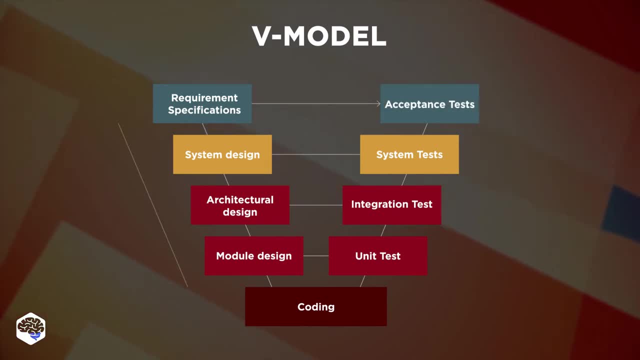 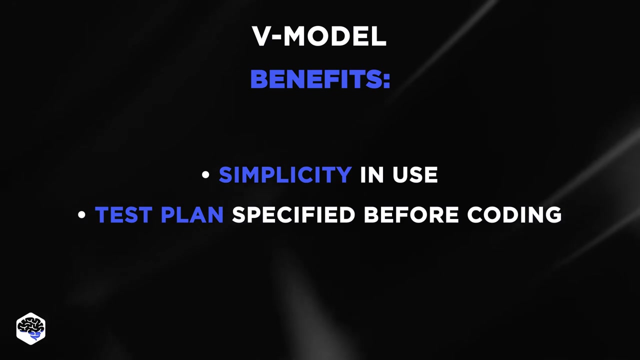 The V-model breaks down the testing phase into detailed steps to ensure the validation and verification process. According to our team's experience, the V-model is rarely used these days. V-model benefits include simplicity in use. the test plan is specified before coding. real-time error tracking. defined user role in the. 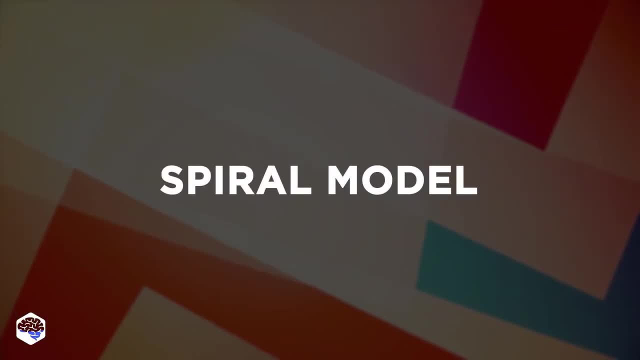 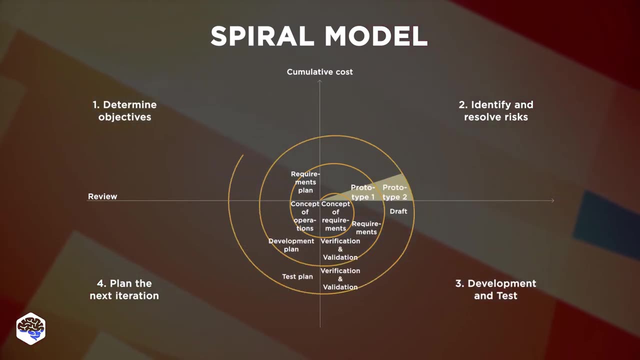 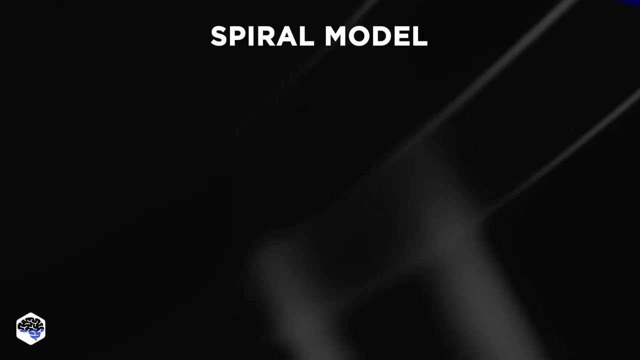 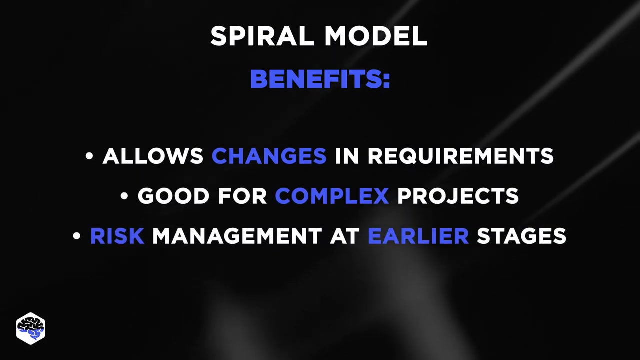 verification phase. and finally, the spiral model. This methodology focuses on risk analysis and spirals development loops. It combines both linear and iterative approaches. Each spiral addresses one single activity of software development. The spiral model has the following benefits: It allows changes in requirements. good for complex projects. ability to manage risks. 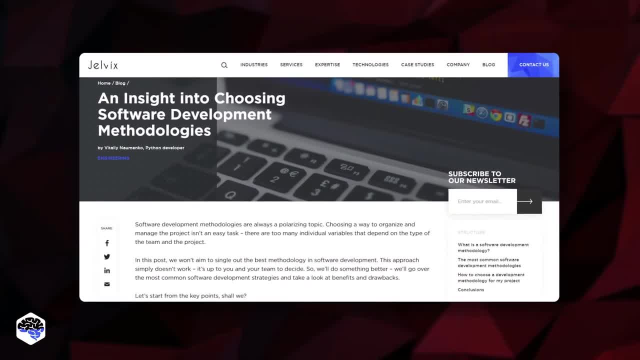 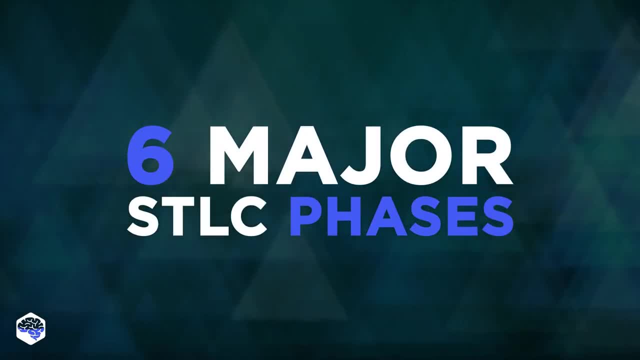 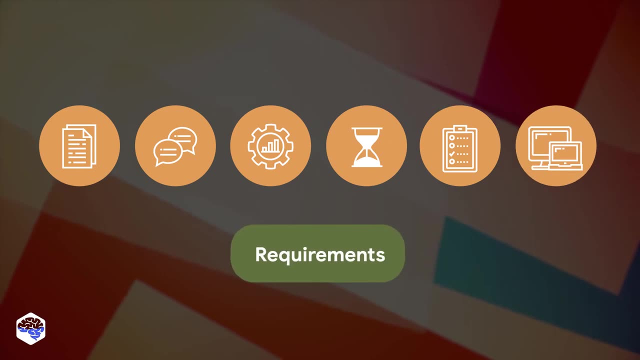 at earlier stages. Would you like to learn more about software development methodologies? Check our guide in the description box. Let's now review the process of software testing lifecycle, Phase 1. Requirements Analysis. After product requirements are set out, Jelvik's testing teams try to evaluate. 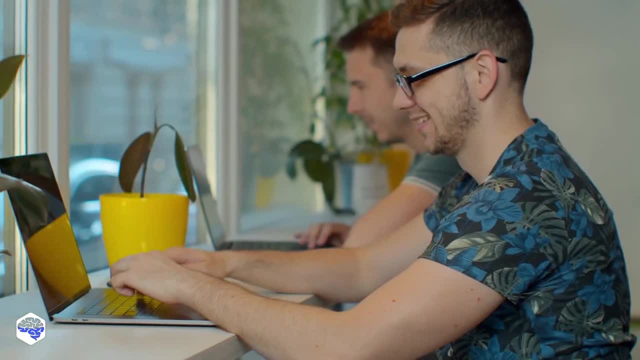 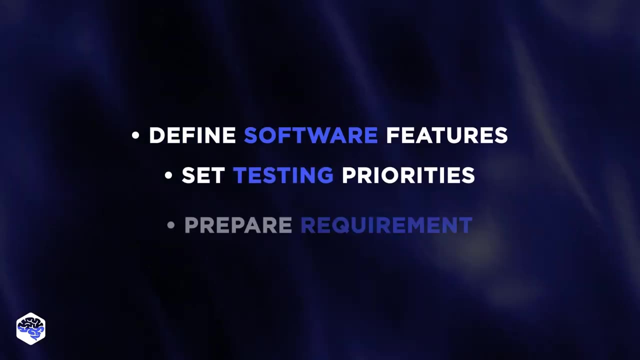 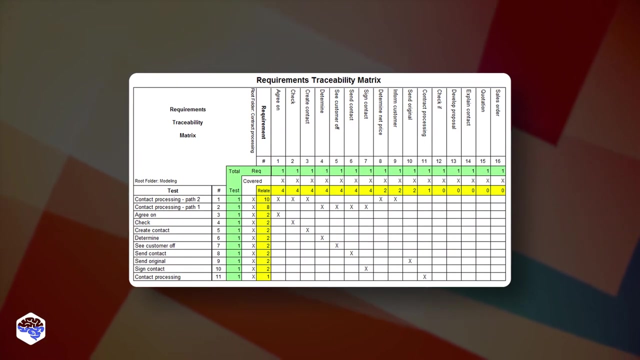 this information and ensure that it works for the project. Requirement analysis includes the following activities: Defining software features, Setting testing priorities, Preparing requirement traceability matrix RTM. It is used to track the requirements and to check if the current project requirements are met. And, finally, we 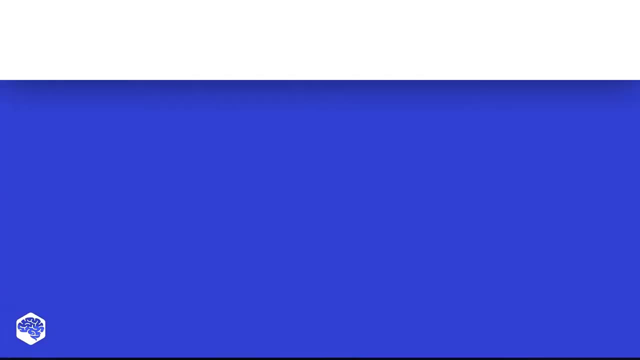 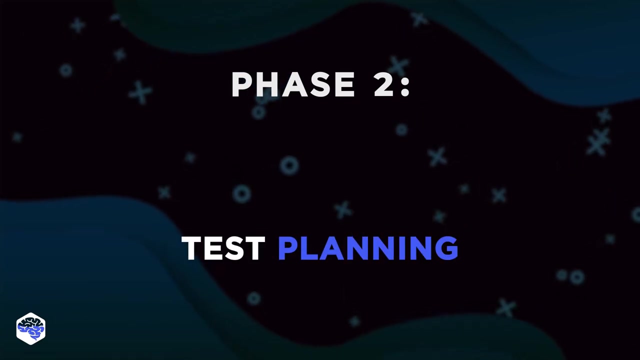 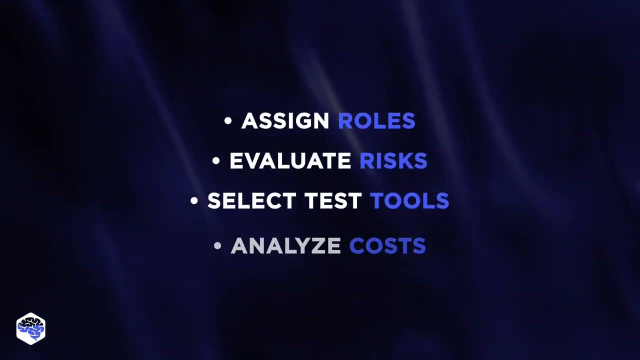 perform identifying the testing environment details. Deliverable of this stage is requirement traceability matrix. Phase 2. Test Planning: Key activities in this stage include assigning roles and responsibilities, risk evaluation, test tool selection and cost analysis. Deliverables of this stage are effort. 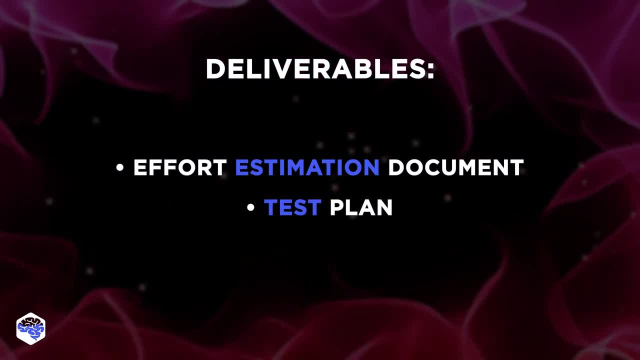 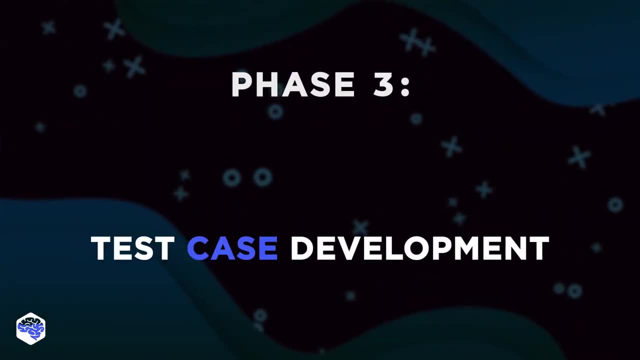 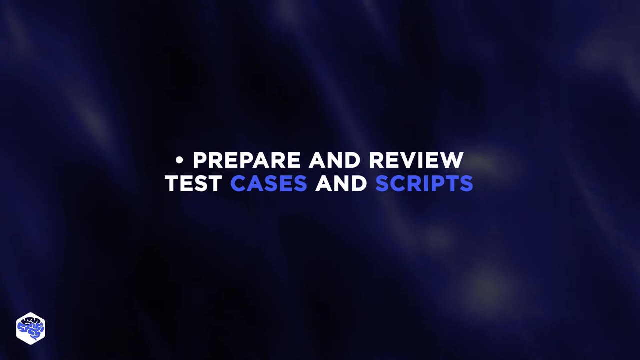 estimation document and test plan strategy document to identify what we are testing, how and what are our outcomes. Phase 3. Test Case Development. At this stage, our team prepares and reviews test cases, automation scripts and creates test data, Obviously deliverables. here are test cases and scripts and test data. 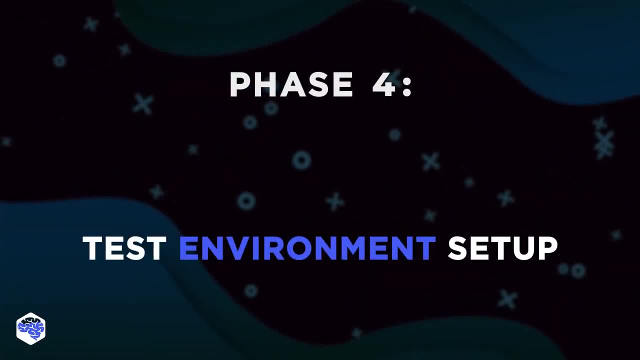 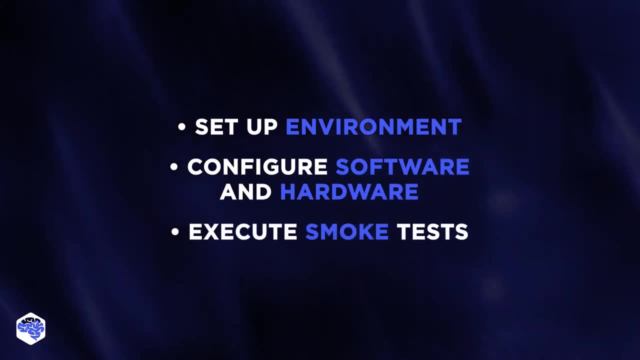 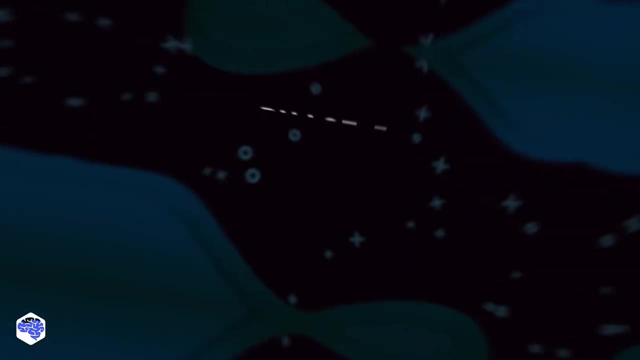 Phase four: test environment setup. Once software build is deployed, we execute environment setup, software and hardware configuration and smoke test execution. As a result, we get the environment ready with test data set up and smoke test results. Phase five: test execution.